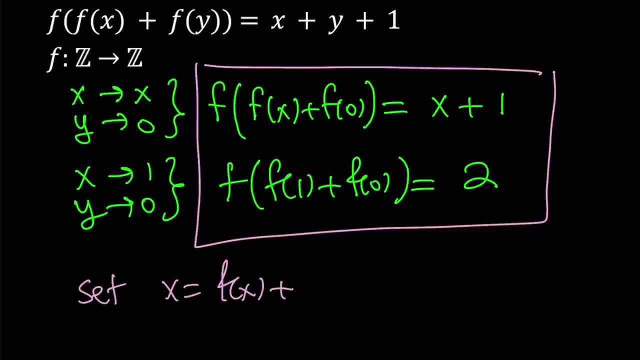 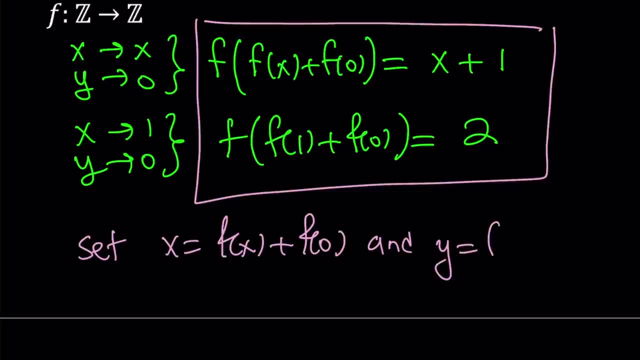 x equal to f of x plus f of 0.. So f of 0 in this case is a constant, And we're going to set y equal to f of 1 plus f of 0. And when we make these replacements in the original equation, this one: 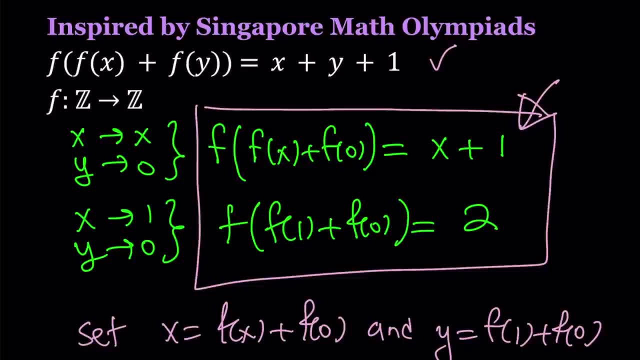 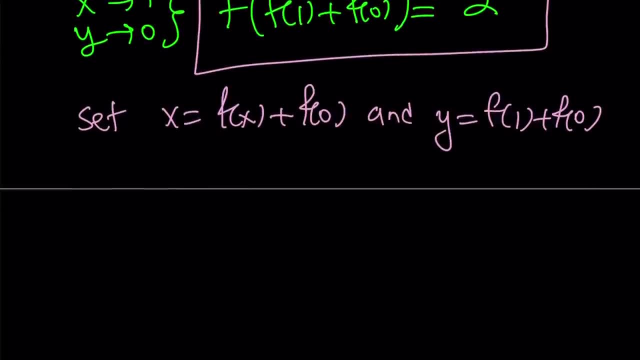 we're going to be able to take advantage of these two equations. So that's the plan. all right, So let's go ahead and do the replacements and see what we get from here. We're going to be getting f of f of f of x, plus f of 0. So that basically just replaces the x. So we have f of f of x. 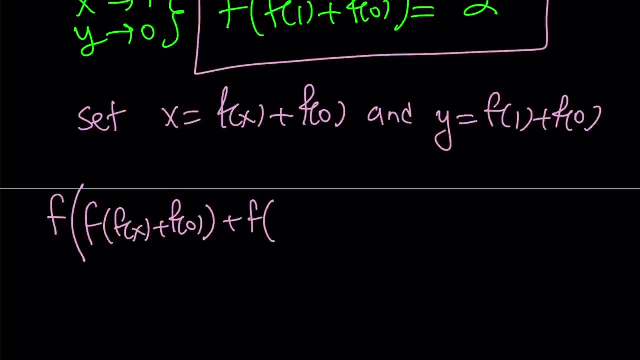 plus f of y, And y is going to be replaced with f of 1 plus f of 0. Awesome. So this is f of f of x plus f of y, And this is going to equal by the definition given to us we're going to set it. 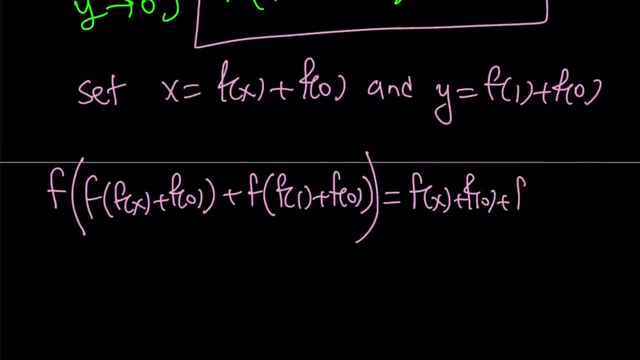 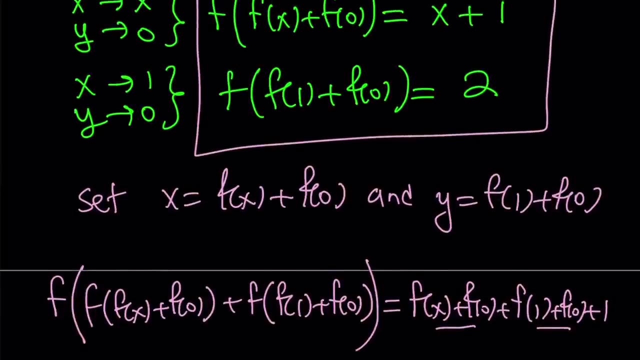 equal to f of x plus f of 0 plus f of 1 plus f of 0 plus 1.. Awesome, So this is our x value and this is our y value. Now notice that we have a value for both of these: F of f of x plus f of 0. 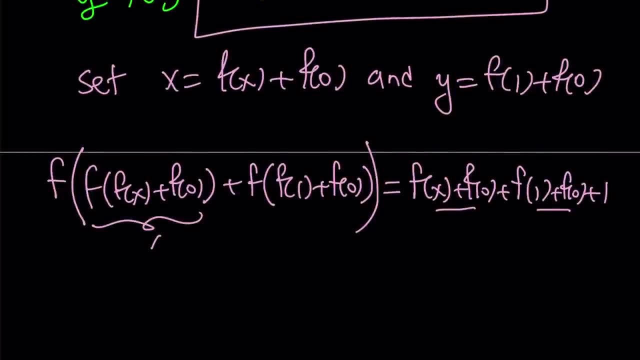 is equal to x plus 1., So we can replace this with x plus 1.. And we can replace this with 2.. So we can replace this with 2.. And we can replace this with 2.. And we can replace this with. 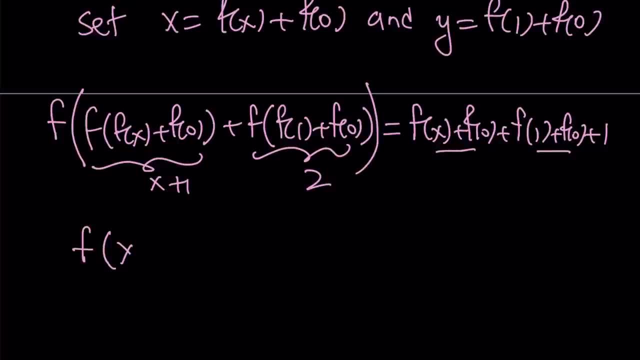 2. that gives us the following: f of x plus 1 plus 2, which is f of x plus 3, and on the right hand side we get the following: f of x plus f of 0 plus f of 0 is just going to be 2 times f of 0. 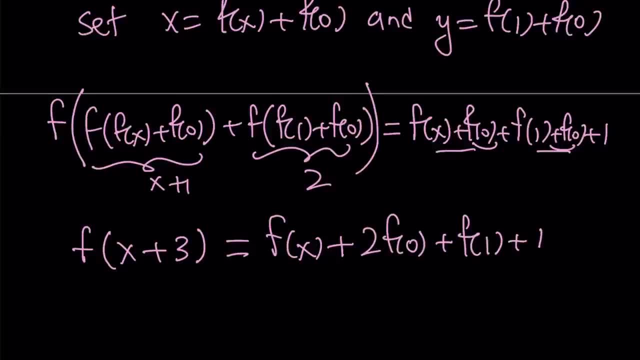 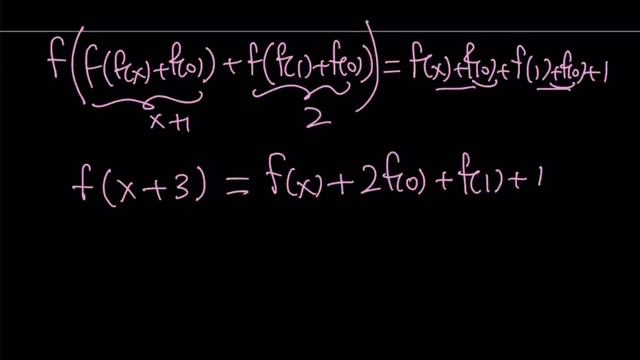 plus f of 1 plus 1. so remember: f of 0 and f of 1 are both constants. therefore this whole thing can be called a constant. so let's go ahead and do that: 2 f of 0 plus f of 1 plus 1. let's go ahead. 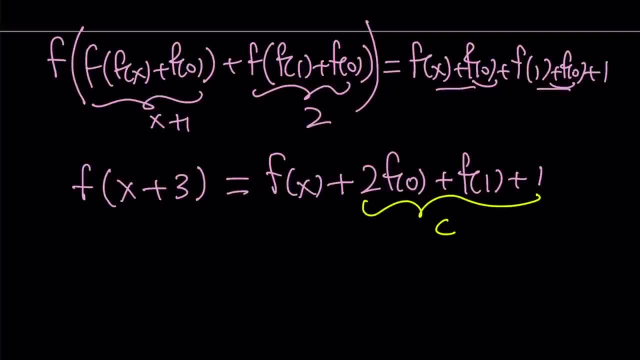 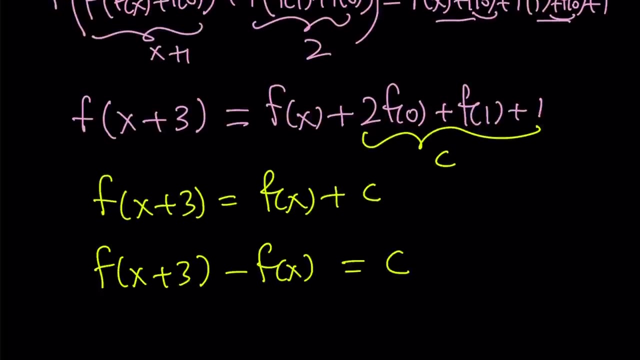 and call that c, where c is a constant. so this gives us a really nice equation: f of x plus 3 equals f of x plus c, c being a constant. we can go ahead and put f of x on the left hand side and get a really nice equation. now remember, f is defined from integers to integers. 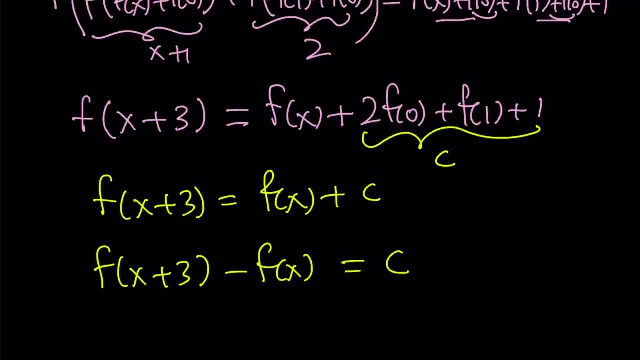 and c is a constant. so what is that supposed to mean? the difference between these terms that are like three of them, are the same. so f of x plus f of 0 plus f of 1 plus f of 0 plus f of 0 plus f of. 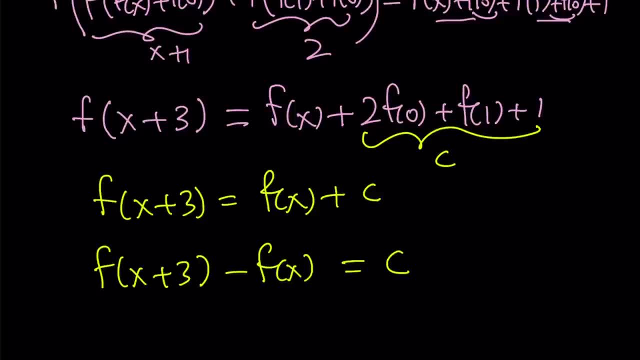 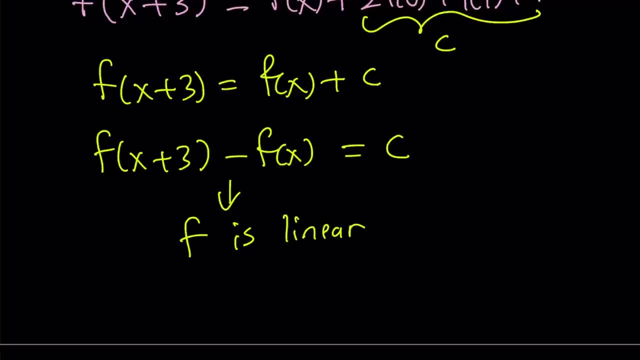 0 is the last part of the equation. so this is the final part and obviously so this. this basically means that f is a linear function. i know some folks already figured out like, okay, looking at this equation, i already know that it's going to be linear, but this is kind of like a more uh, concrete. 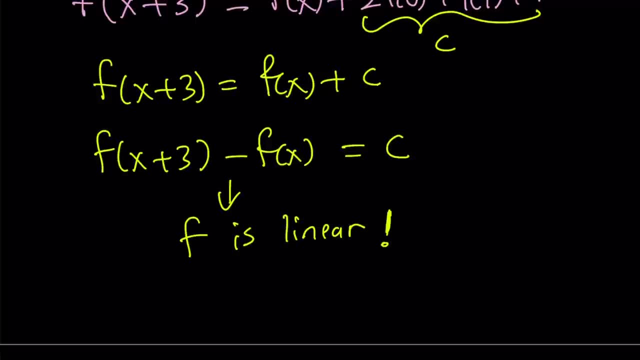 reason for f to be linear, not just eyesight. okay, so f of x can be written as, since it's linear, mx plus b. awesome. and from here we can safely say that f of y is going to be m, y plus b. Remember, x and y are free variables, So don't. 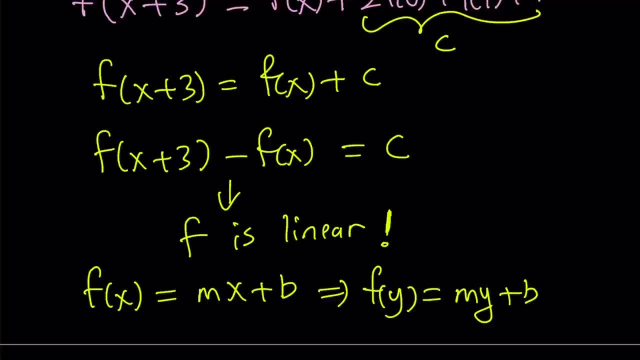 think about it as f of x equals y. It's not the same thing. I know some folks are saying, okay, use a different variable, But a lot of times with functional equations- well, with integers, I guess a and b could be more appropriate, But anyways, I just used x and y. 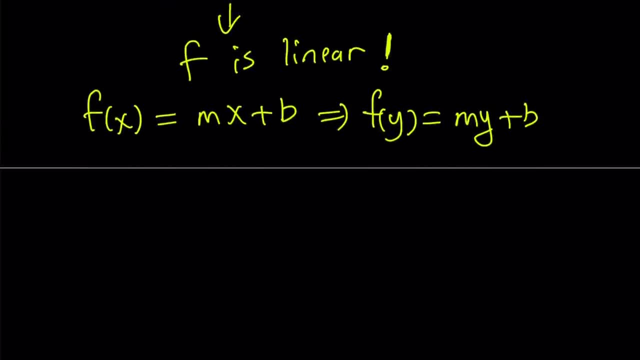 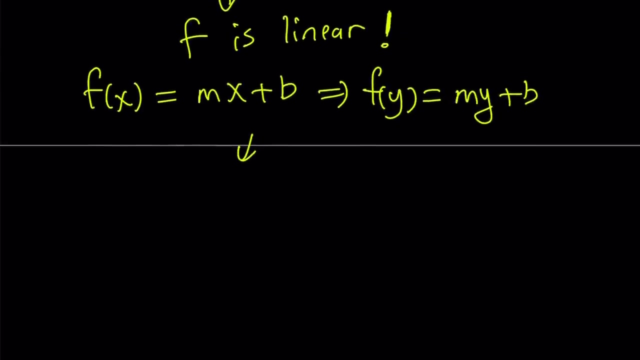 Sorry about that if that bothers you. So f of x. we assume that. well, we didn't assume. I guess we can assume it's safe to assume that f is going to be linear. So now we're going to substitute- Okay, we're going to substitute this into the original equation. And because we want 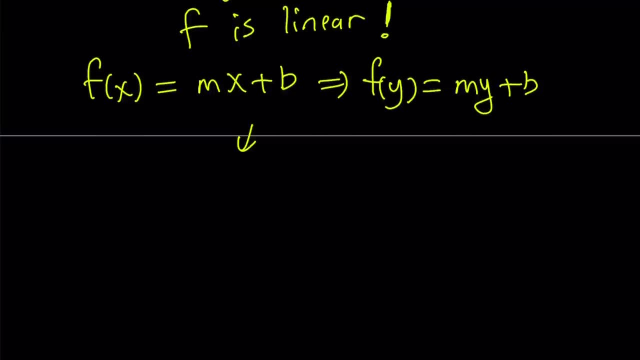 to determine the m and b values, if possible. All right, great, And this is going to allow me to use one of the jokes, Anyways. so remember, our original problem was f of f, of x plus f of y equals x plus y plus one. So if you go ahead and substitute this into the original equation, you're going to get the original equation. So if you go ahead and substitute this into the original equation, you're going to get the original equation. So if you go ahead and substitute both of these into this equation, you're going to get. 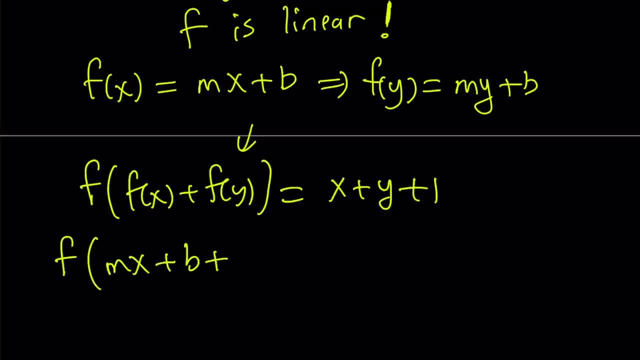 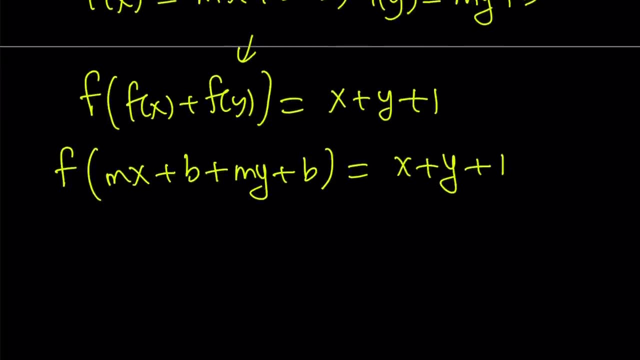 f of m x plus b, and I'm going to take show my work here: plus m y plus b equals x plus y plus one, And then I'm going to add these two together, m x plus m y, and write it as f of m times x plus. 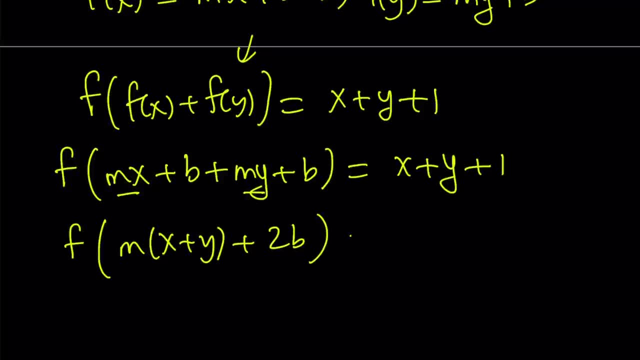 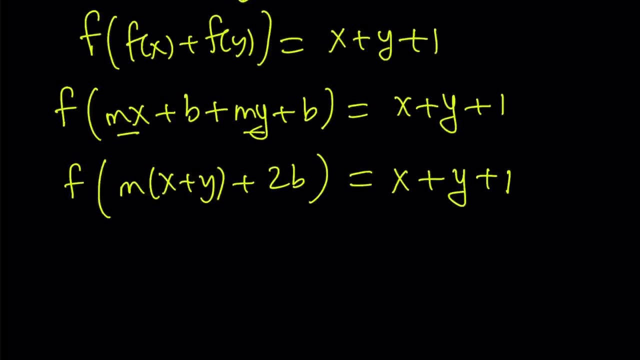 y plus 2b, 2b or not 2b? Okay, that's the problem. Great Yay, I got 2b again. So now using the definition of f again one more time. right, we said that f is written as m x plus b. 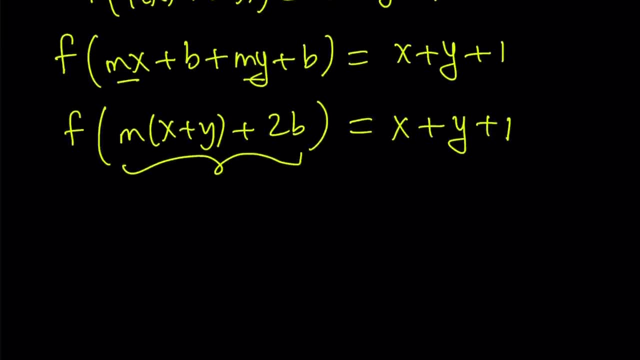 So let's go ahead and replace x with this. So in other words, multiply the argument by m and add b, So it's kind of like m times this quantity plus m equals x plus y plus one. Obviously, this equation should be true for all x, y values that. 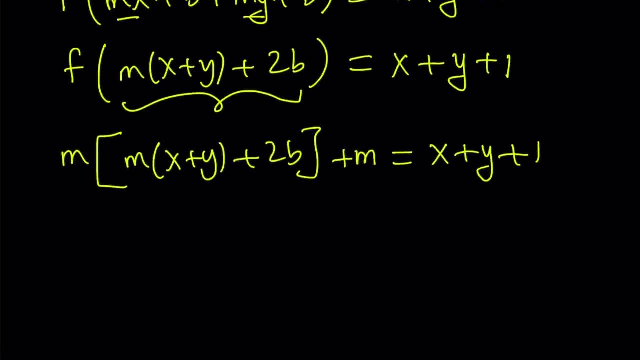 are in the domain. So we're going to get kind of like a polynomial equation. All right, great. So this gives us m squared times the quantity x plus y. The reason why I don't want to distribute it is because I have x plus y on the right hand side, So it kind of works nicely. And then from here we get 2mb. 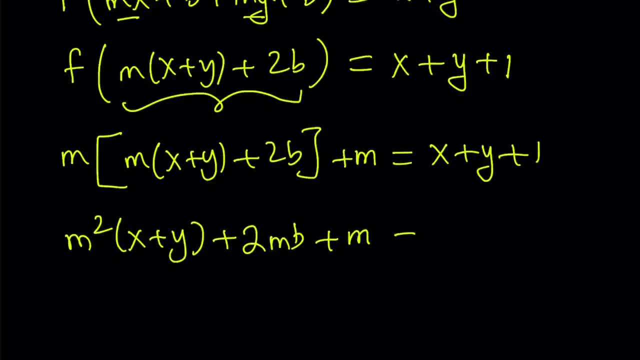 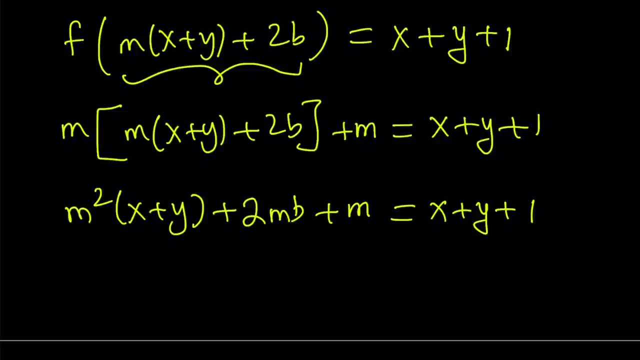 plus m, And that equals x plus y plus one. So now, comparing these two sides, or the equation side by side, we notice that the coefficient of x plus y on the right hand side is one. And since this is true for all x- y values in the domain, 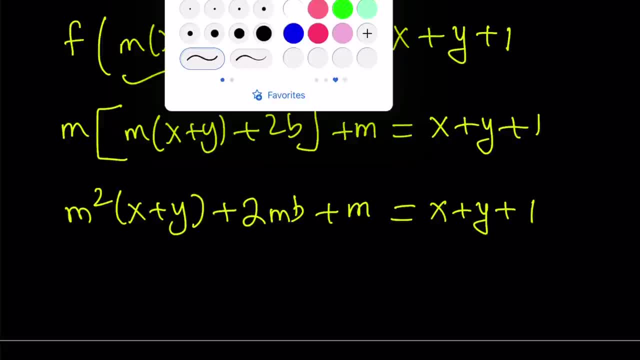 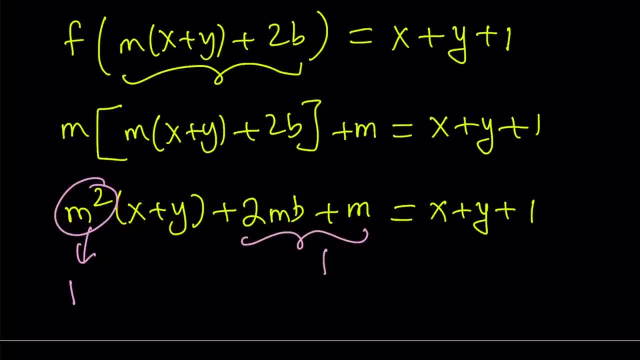 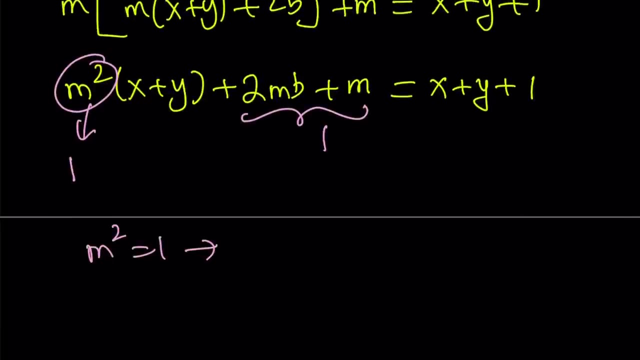 this implies that m squared equals one. Okay, great. So m squared equals one. And also this implies that 2mb plus m is equal to one. So we get a system of equations. Let's go ahead and solve this system. So m squared equals one implies m equals one or m equals negative one. 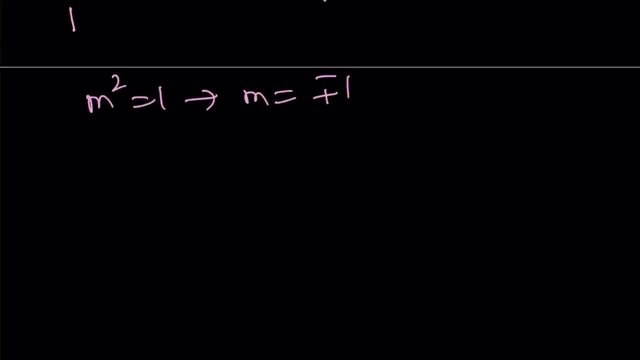 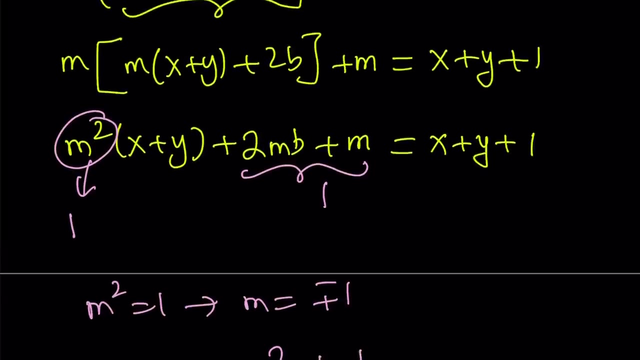 So m equals plus minus one. So we can safely say that m equals one and 2mb plus b, which is the. by the way, it's not 2mb plus. okay, I made a mistake there. I'm like: 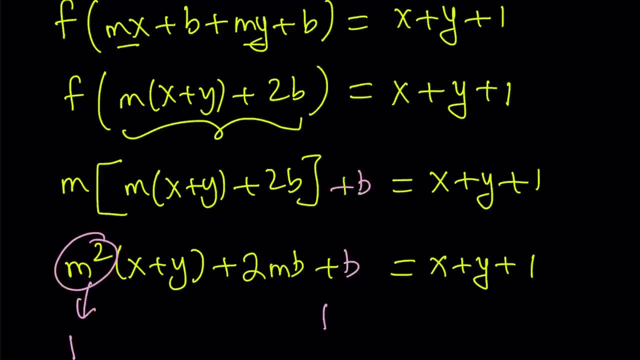 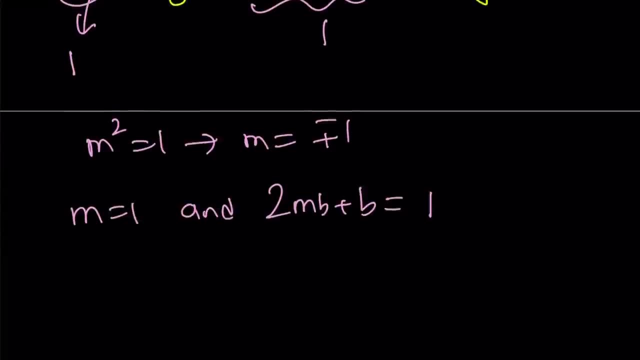 what is going on here? This is supposed to be b. I apologize, That is not m, So this needs to be one. Therefore, 2mb plus b needs to be one. Okay, great. So now from here we get the following: 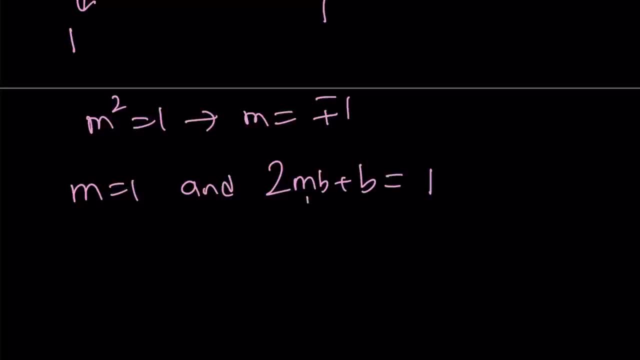 If m is equal to one, you can kind of plug it in here. you get 2b or not 2b. 2b plus b is equal to one. 3b equals one And that means b is equal to one. So 2b plus b is equal to one. So 2b plus b.